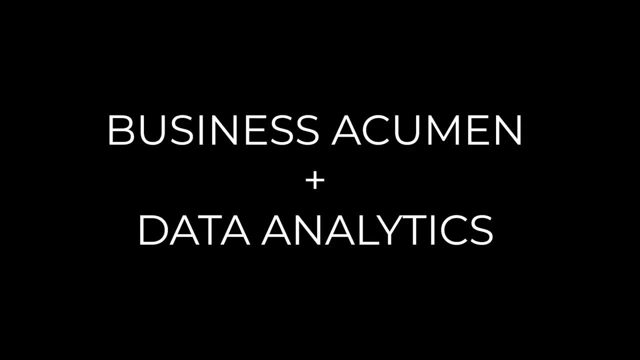 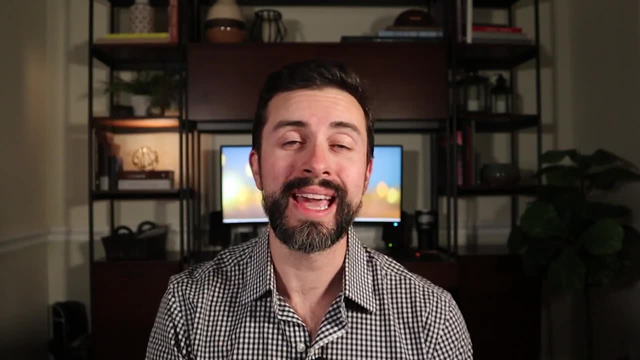 but they're really looking for now experts in data analytics. After all, that's a really big part of the business. So if you're looking for a good business, you're looking for a good business decision-making equation. So in this video, I'm going to give you a brief walkthrough. 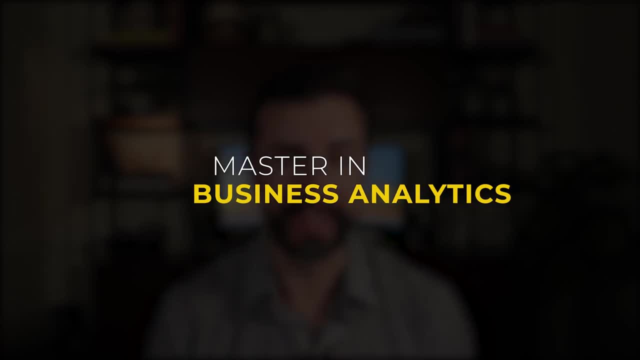 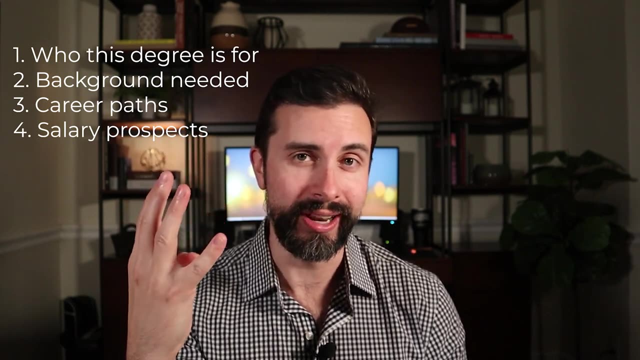 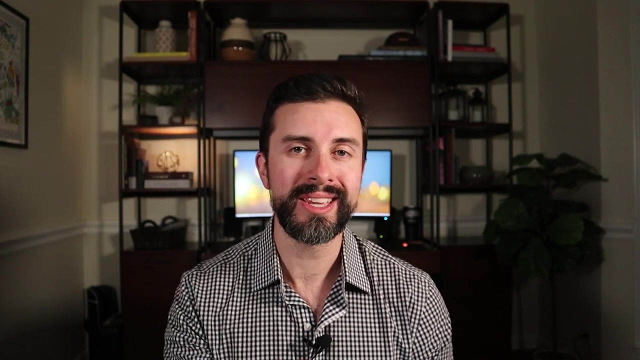 of the master's in business analytics degree who this is for, what kind of background you might need, as well as career and salary prospects after graduating. So let's get to it. What is a master's in business analytics? The degree is meant to equip students with the ability. 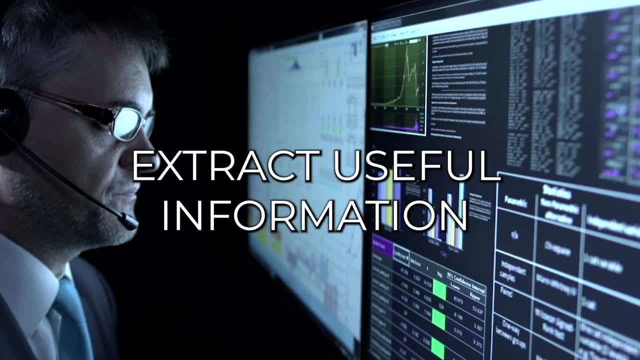 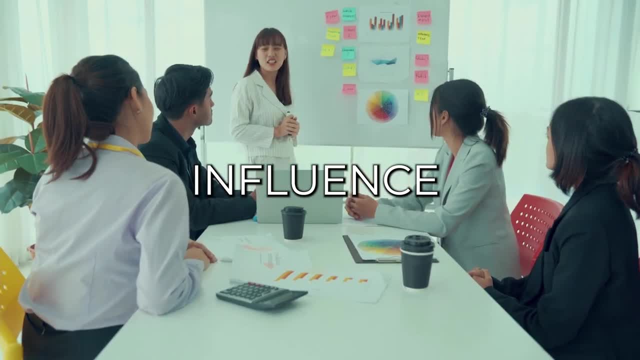 to gather data, organize it, extract useful information from it, influence others through strategy and to be able to do the right thing. So if you're looking for a good business, you might want to think of storytelling with data, You might think of data visualization. 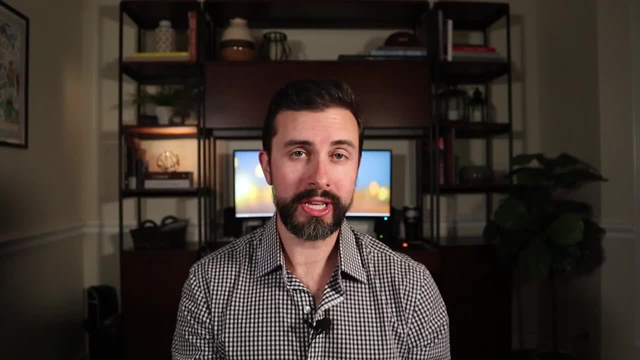 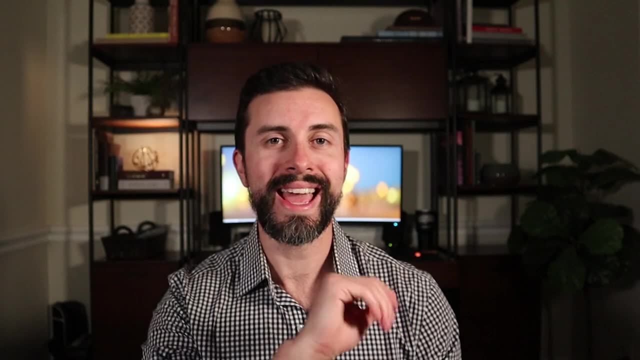 techniques to help tell a compelling story And ultimately you use that to inform a good business decision. By the way, this skill, my friends, happens to be useful in just about any role in any organization, at any company. For example, think of supply chain when you 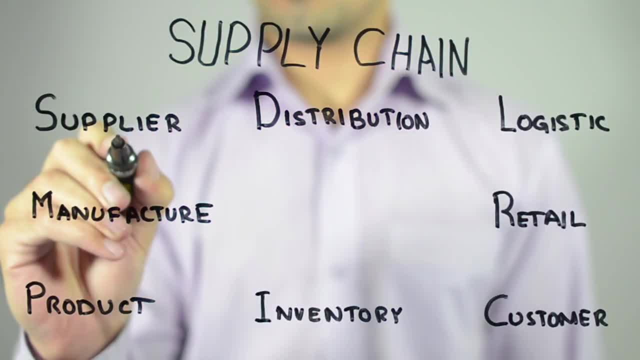 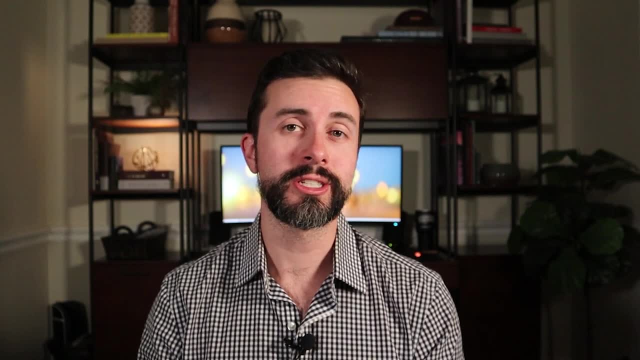 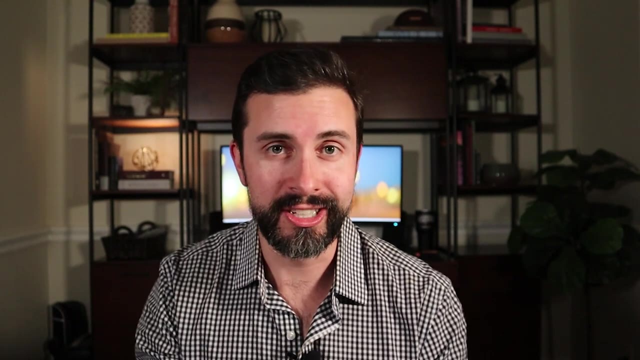 have to have accurate forecasts on when to place orders to manufacturers so that you get product in the time that customers are actually going to order also needs to be accurate because you also don't want products sitting in a warehouse for an excessive amount of time, incurring additional storage costs. 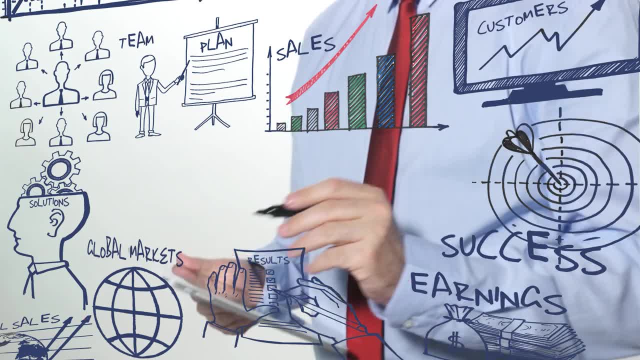 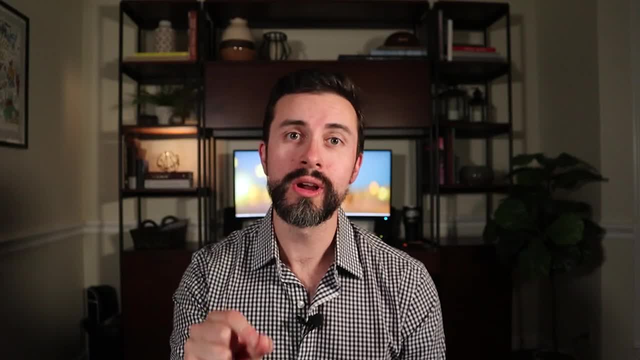 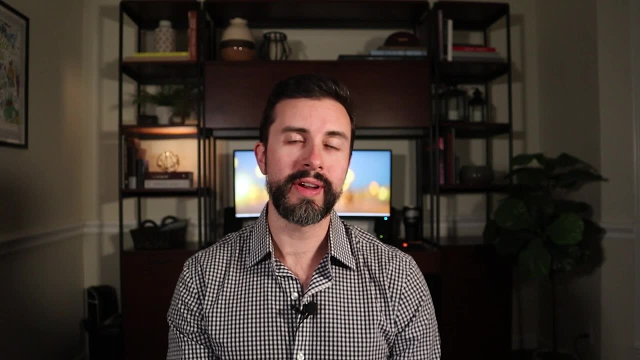 you also might think of marketing when analyzing different actions that the company is taking to drive traffic to a website or drive sales. data analytics is at the core of what makes an optimal business decision and informs what to do next. so what background do you need? this is going to vary by University, but from 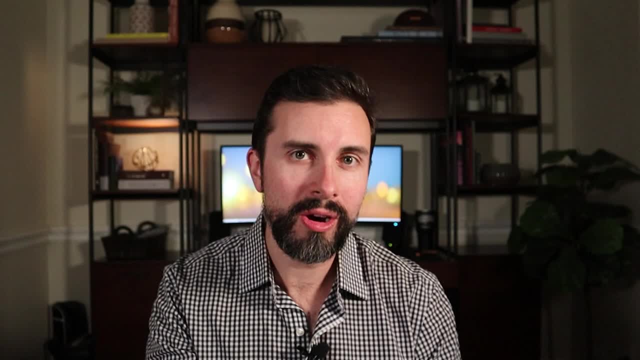 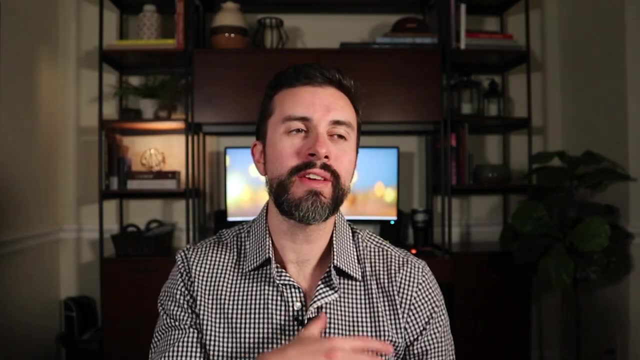 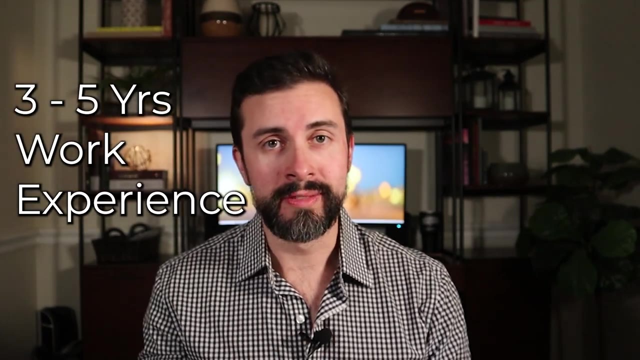 what I've seen, there aren't really any hard definitive requirements. most of these programs are designed for people earlier in their careers, but you will want to have a few years of work experience under your belt. I normally recommend anywhere from 3 to 5. it's also what I happen to recommend for anyone. 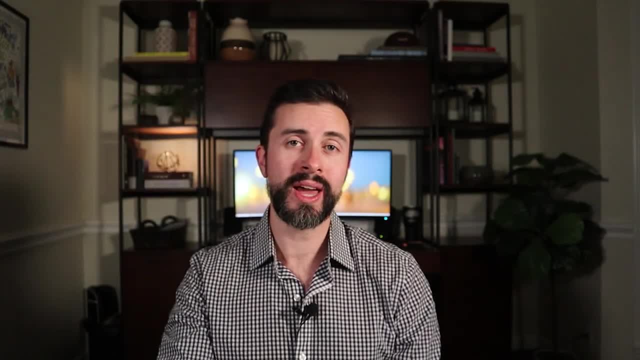 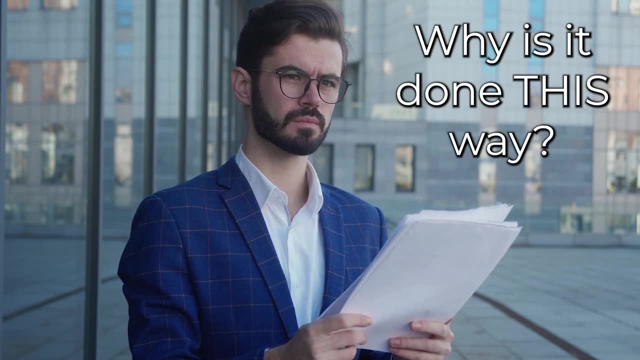 thinking about an MBA program, but my reason for that is so that you are aware of how companies operate and it can lead you to asking questions about why things are done a certain way, or you even do that to yourself in the process and if you're not sure what to do next. 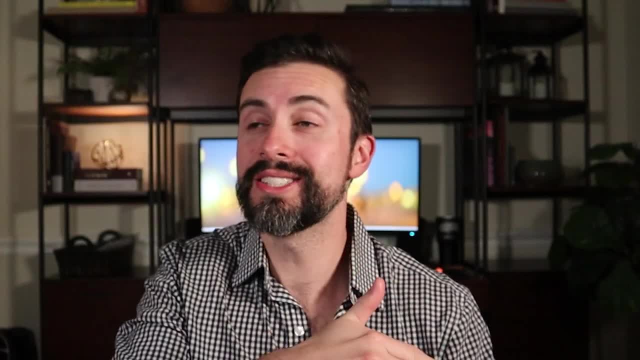 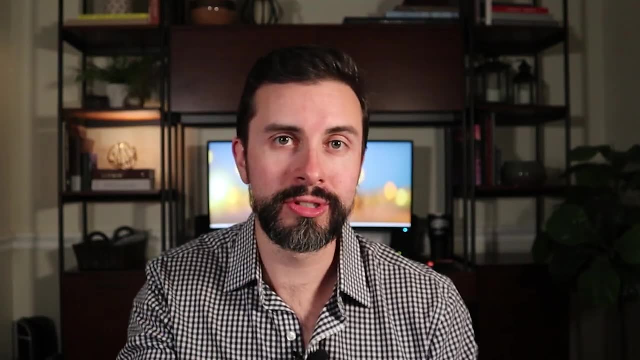 better questions like: does it have to be this way? Is there a better way, So that, as you have that perspective, you can go into these degree programs and you're almost immediately able to imagine and think about how you would apply what you're learning in class to a real world? 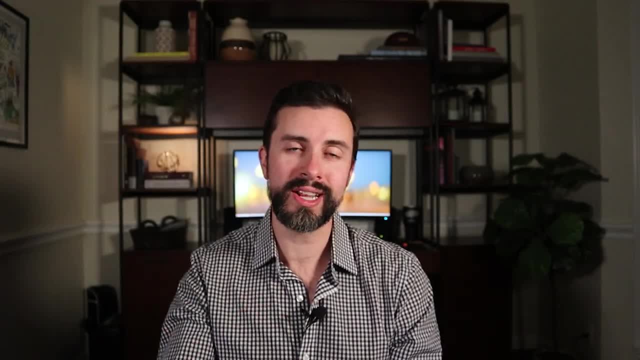 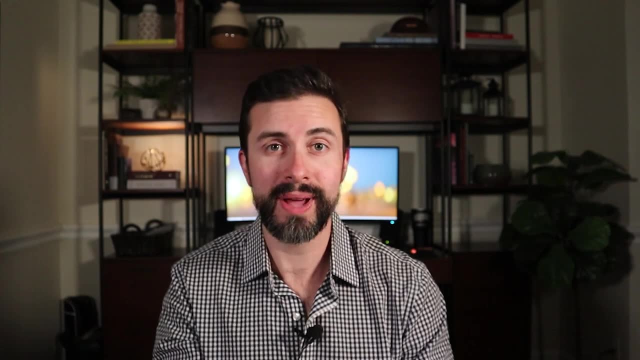 business problem. It just gives you so much more context on what it is that you're learning and why it matters. And because you're able to make those mental connections, you're going to remember the material far better. Now, in addition to simply the number of years of experience, I'd also 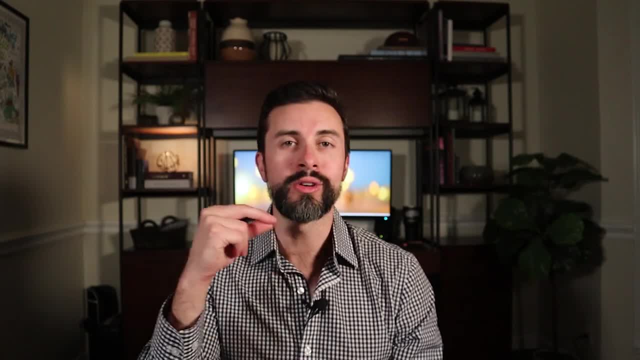 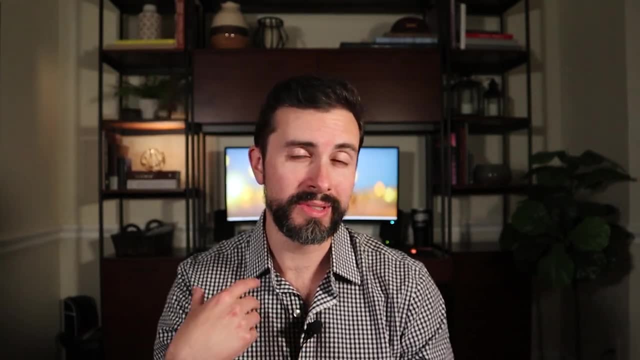 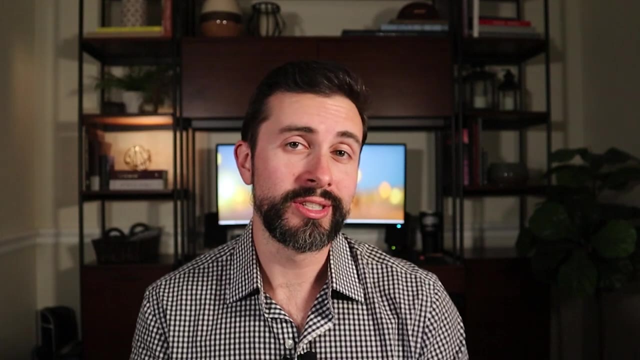 recommend that either in your work experience or in your education background, that you have some evidence of quantitative knowledge At work. maybe you've done some data analysis where you've used something like Excel to do some kind of modeling. Maybe you've used some data visualization software. 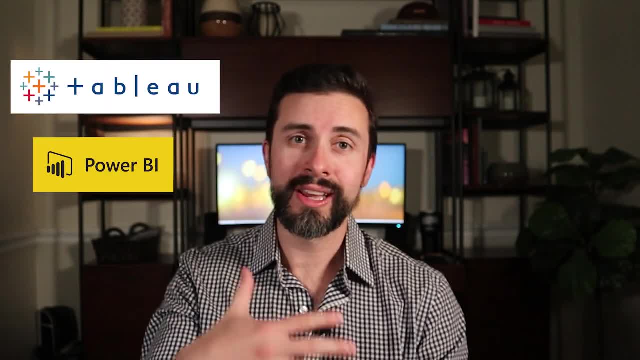 like Tableau or Power BI to look at data and make a decision. But if work hasn't presented you those opportunities, you're not going to be able to do that. So if you're able to do that, then you're going to be able to do that. So if you're able to do that, then you're going to be able to do that. So 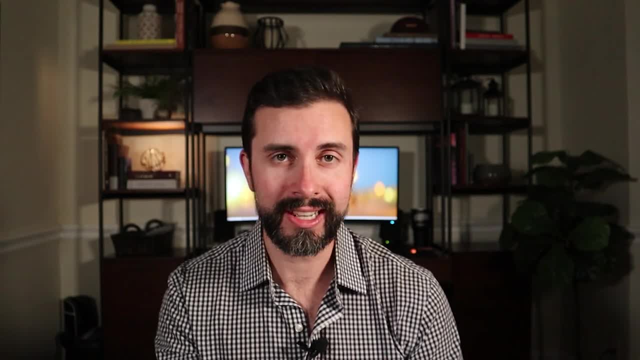 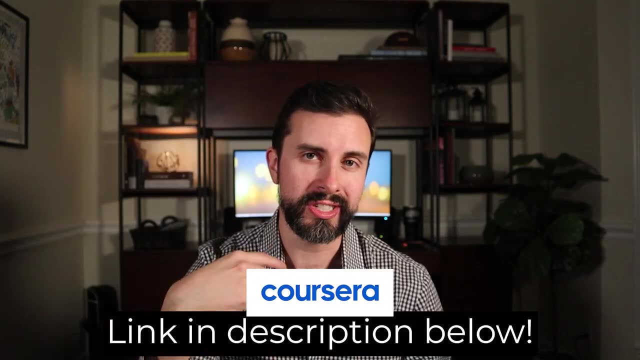 there happens to be some really affordable and flexible education options that will help you bridge that gap. Make sure to check out the link below in the description to Coursera. It's a platform that I've used for many years and recommend it highly. There you'll find many 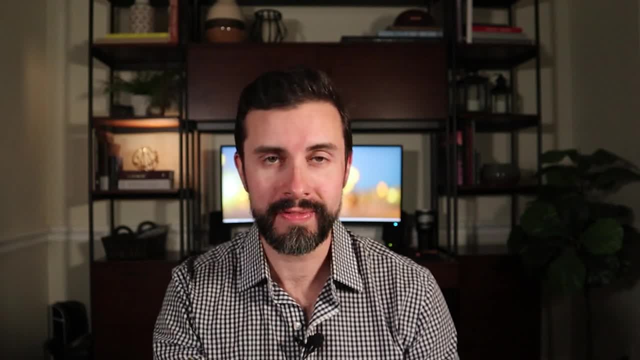 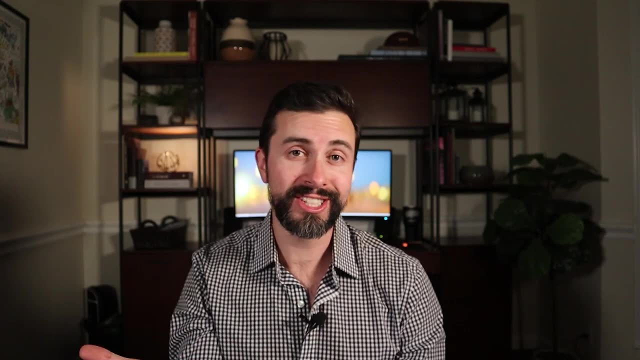 business analytics courses that you can take and you can earn a certificate by completing it, But this is going to help you become more familiar with some of the topics that you would encounter in a full-fledged business analytics degree program, Which, by the way, this might actually 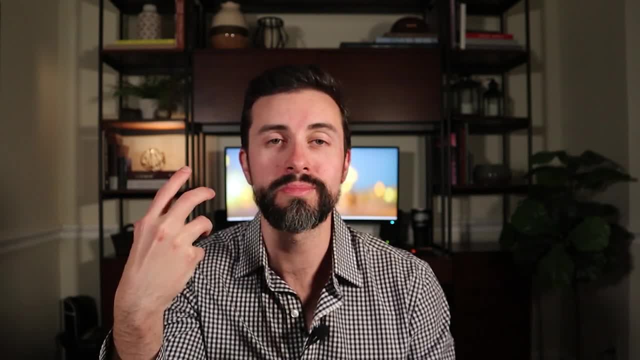 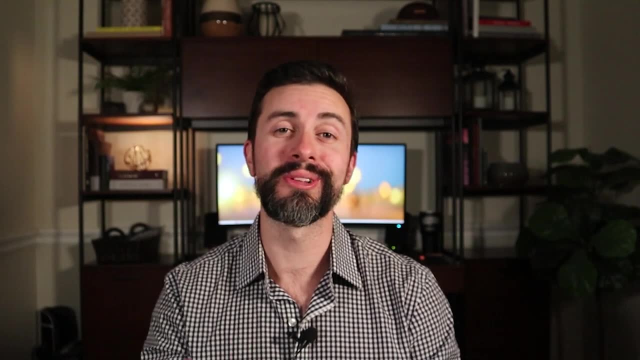 give you some indication as to whether you are serious or would like to pursue the full-fledged degree option. It might turn out that you really do not enjoy the material whatsoever and you find it extraordinarily awful to go through, In which case you might decide this isn't the path I want. 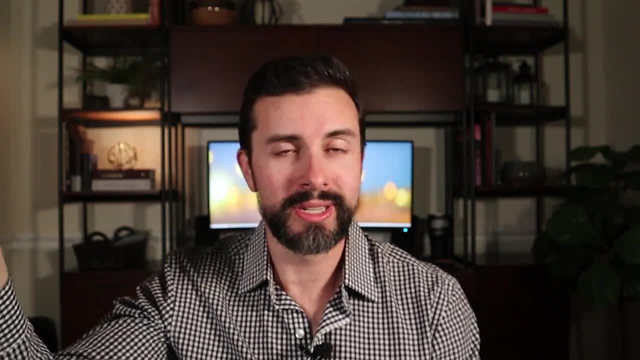 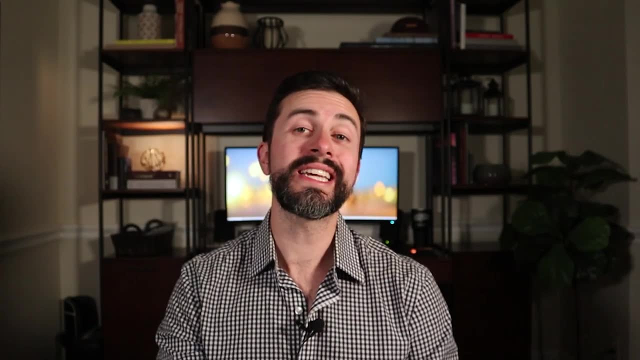 to go down. There's no need in spending a bunch of money on a master's in business analytics degree Now, although the career prospects are quite incredible, which I'll get to in a moment. if you ultimately don't enjoy it enough, you're not going to have to go through a lot of the 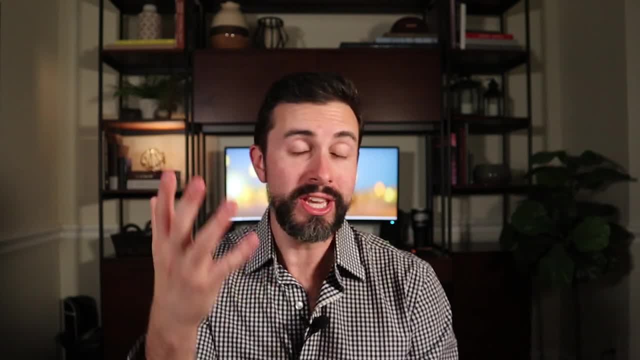 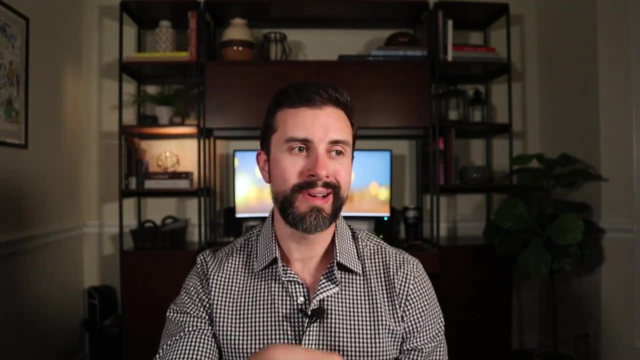 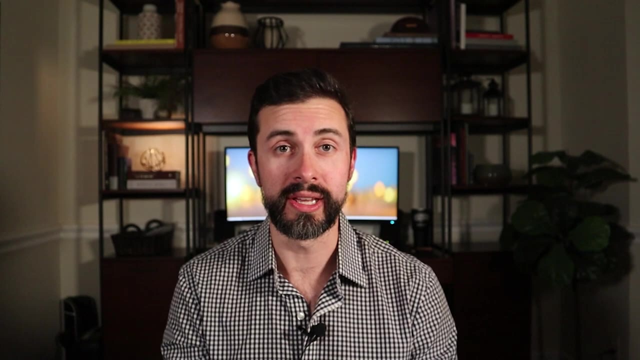 long-term motivation to learn it, be good at it and then have a career in exactly that field that you're studying. One last note that I'll mention as far as a possible requirement- or I would say maybe a nice to have, is some kind of prior experience with programming or coding. Now, 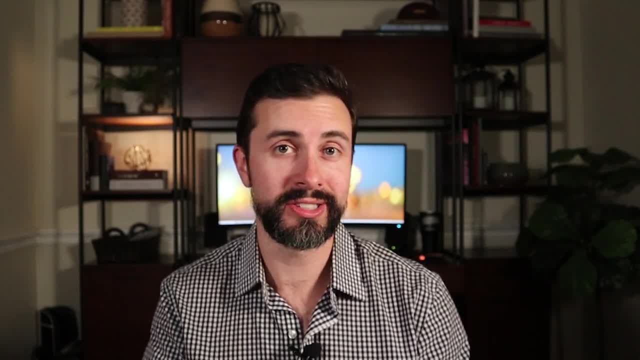 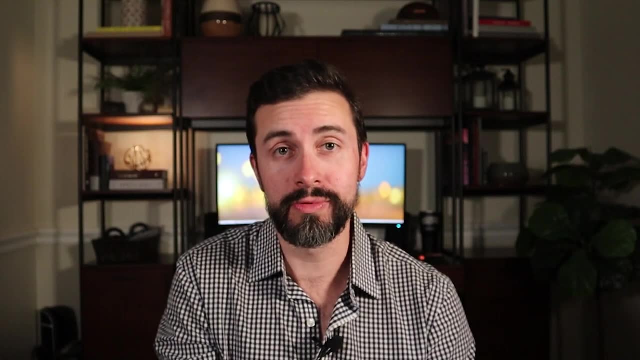 this would be more relegated to perhaps a data science degree, which goes a lot more in that direction, But for a business analytics degree it can be quite helpful. Every school will have some kind of curriculum in terms of how deep they go with requiring you to do any kind of. 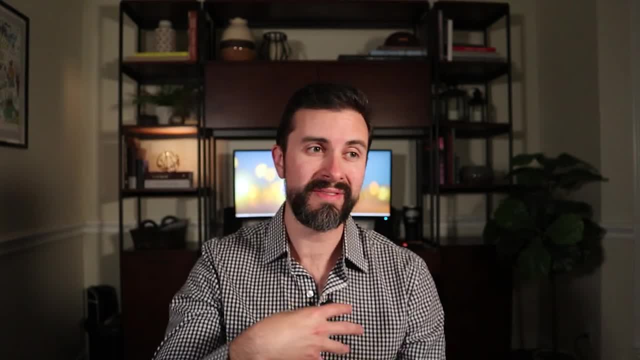 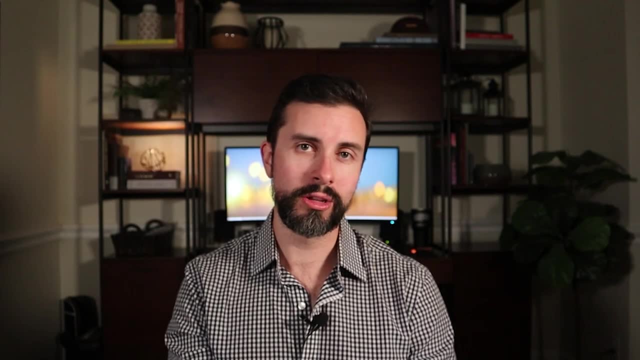 programming or coding. Some degree programs may keep it at a fairly basic level and some of them might get a little bit more in the weeds or a little bit more complex. It all depends. but you'll want to take a look at the specific curriculum of the school that you might be. 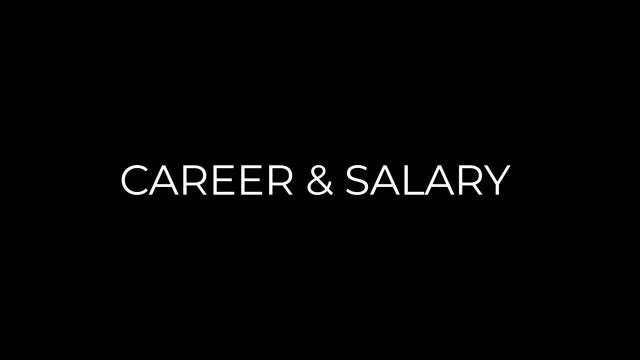 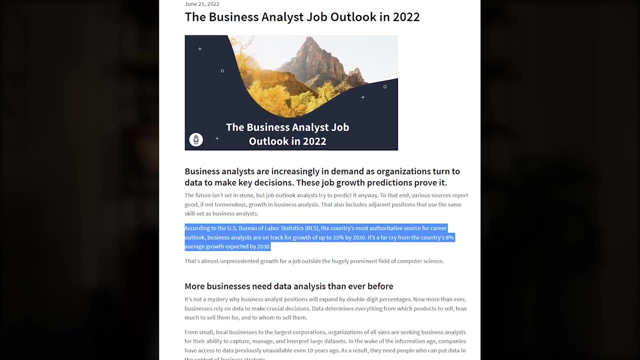 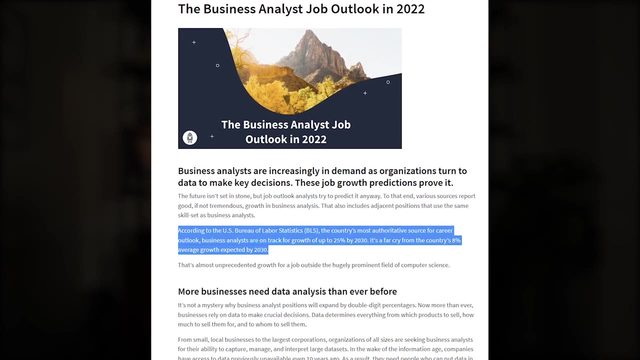 interested in. Now let's talk career and salary prospects, because it is quite compelling. According to the US Bureau of Labor Statistics, business analysts are on for growth of up to 25% by 2030, compared to the US average of 8% growth. Cool thing is. like an MBA. you can take this business analytics degree into just about any industry, any organization, any company. Career prospects, I'd argue, are virtually limitless. This is because you're able to get your foot in the door with a very valuable degree and work your way. 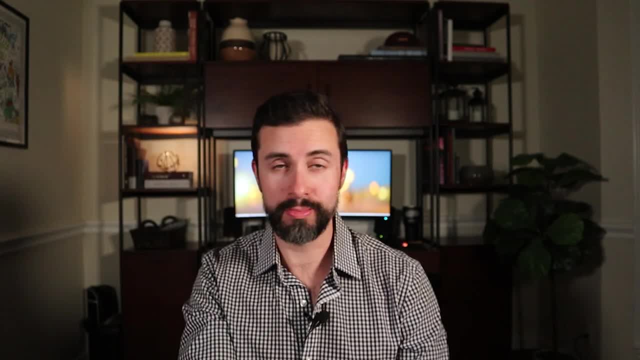 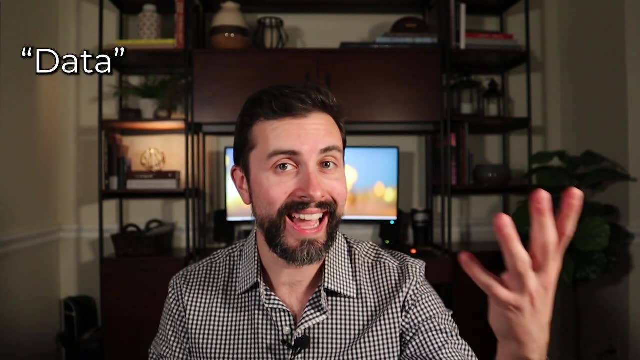 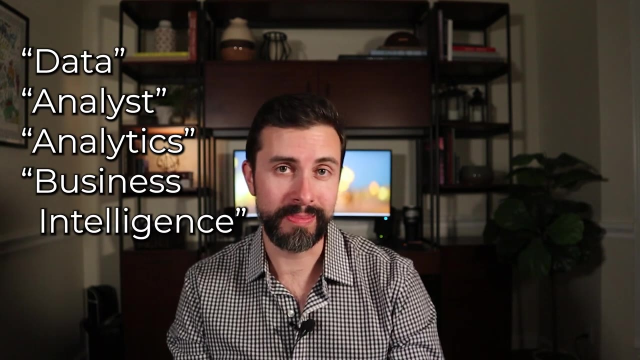 through that company and get some more experience. The hardest part is just getting in. As far as roles that you would be qualified for with this degree, anything that has data or analyst or analytics in the job description or title would be appropriate. Business intelligence is another term that might come up that would also be. 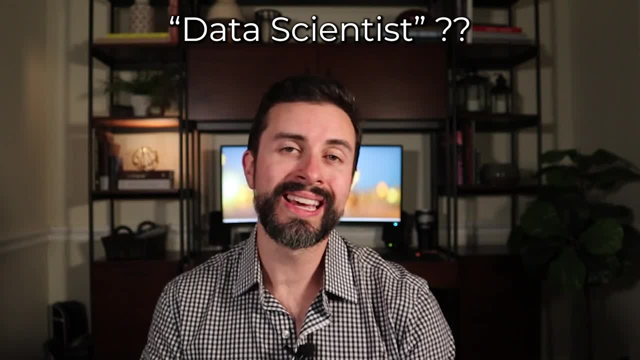 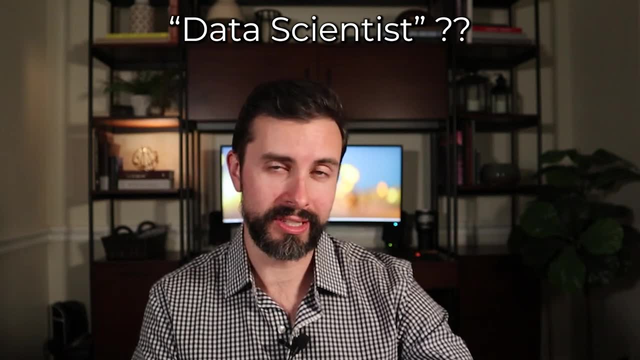 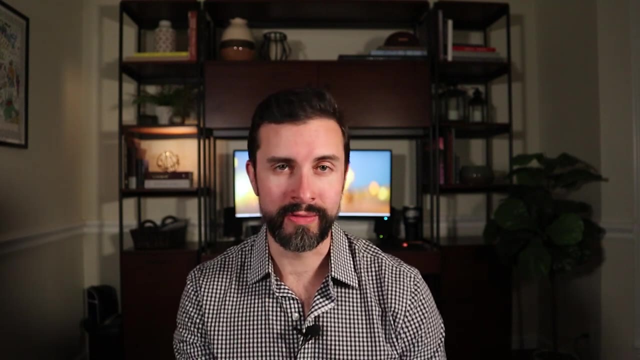 something you'd look into Now. data scientist, in my opinion, is a little bit more of a stretch, but that is also possible depending on really what you learned in your business analytics degree. Now, as far as salary expectations, this one's a little bit more nuanced for a number of reasons, especially when comparing to an MBA. 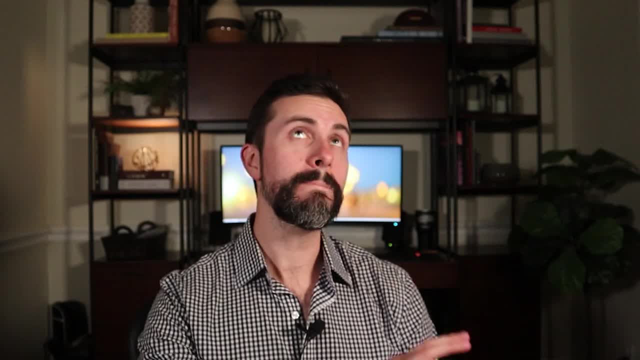 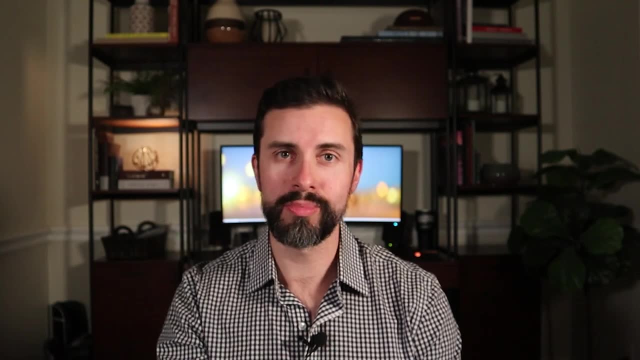 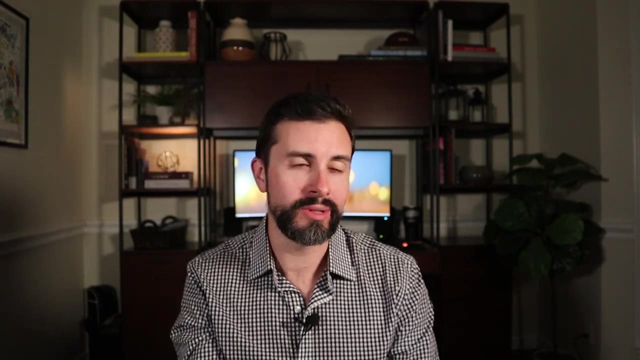 degree First is MBA degrees have been around for much, much longer. There's a lot more data across so many different schools, a lot more data around salary and career prospects, whereas business analytics degrees are relatively new. There's just not as much data that you can go and. 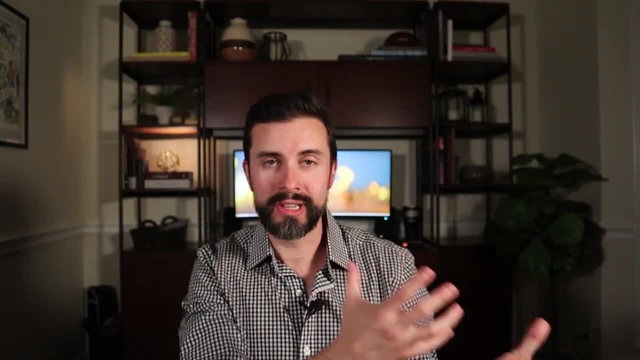 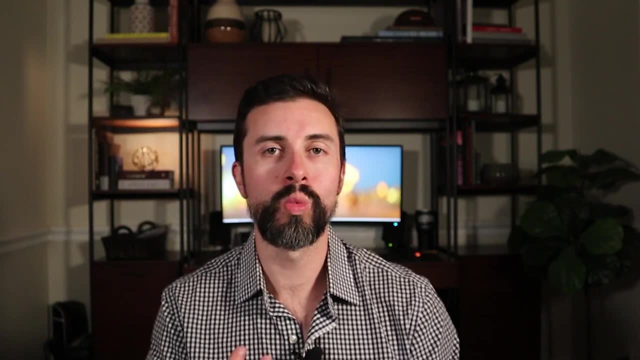 scout to get a broad view or a broad picture of what this degree can do for you On average. Second is MBA degree holders tend to have a little bit more work experience under their belt compared to someone that might be doing the master's in business analytics degree And as 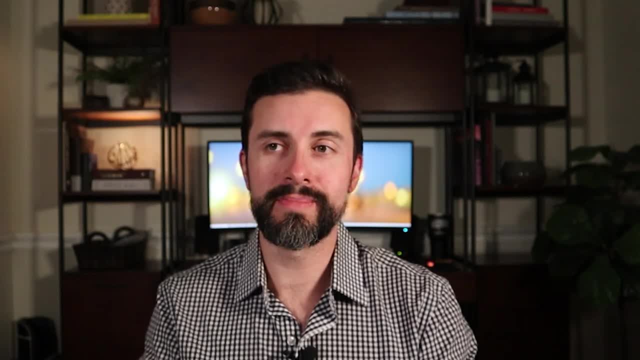 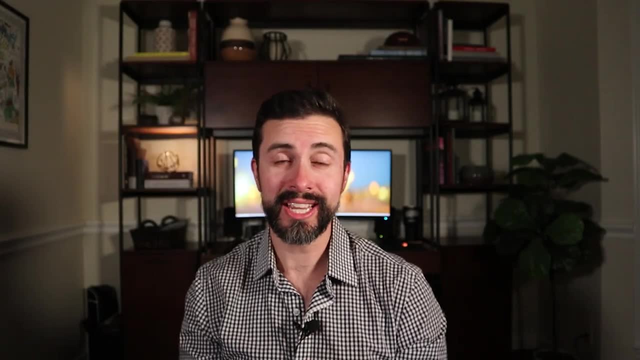 they exit the program and go back into the workforce, the tendency is that they're going to be able to command a little bit of a higher salary for that reason. Lastly, the way that salary expectations are calculated: they vary quite a bit depending on how a particular survey 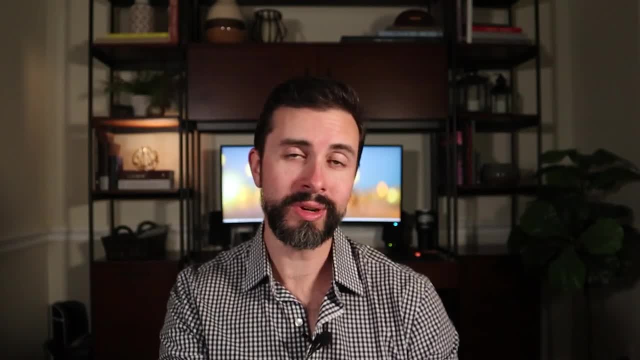 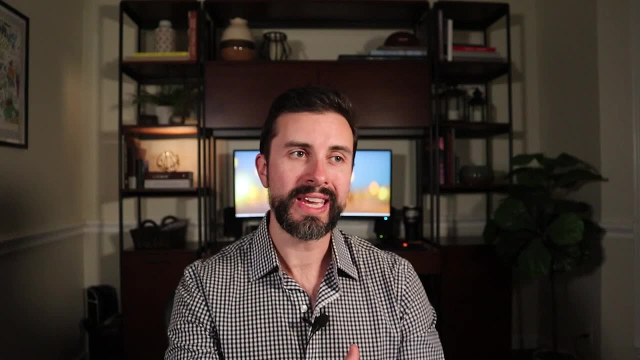 was done. So you're going to see a lot of variation. You're going to see a lot of variation. in fact, if you were to Google it, you would get a ton of different figures for either degree. That aside, I would say quite confidently that if you have a good number of years of work experience, under your belt, I would say, or consider maybe three to five, as I mentioned before, and you have a, an MBA or a master's in business analytics, you can look to six figures. That is an achievable income after graduating with either degree. I will stress: it's not guaranteed. 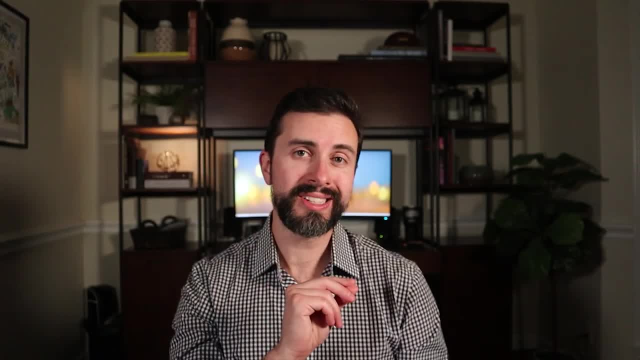 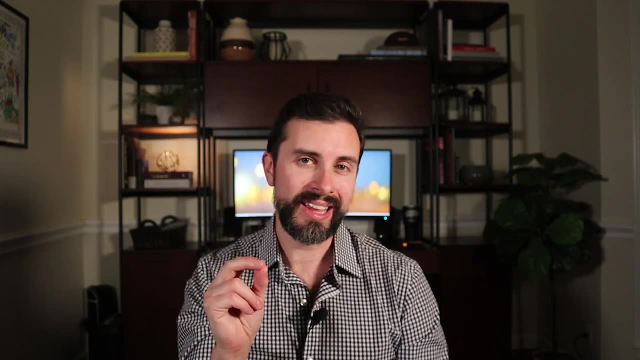 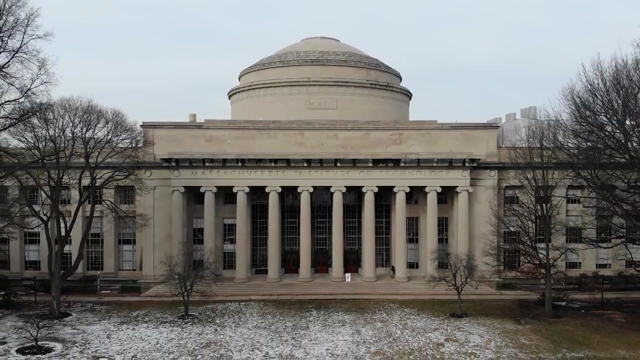 but what I'm saying. it is very much a achievable, But for comparison's sake, let's take a look at one school in particular that offers both an MBA and a master's in business analytics degree, And this happens to be one of the best schools in the world, And that university is MIT. And while we're comparing, 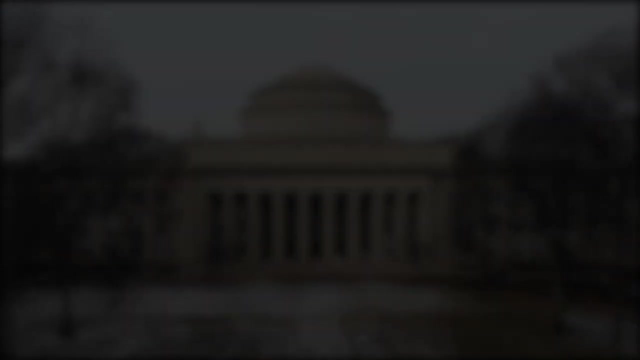 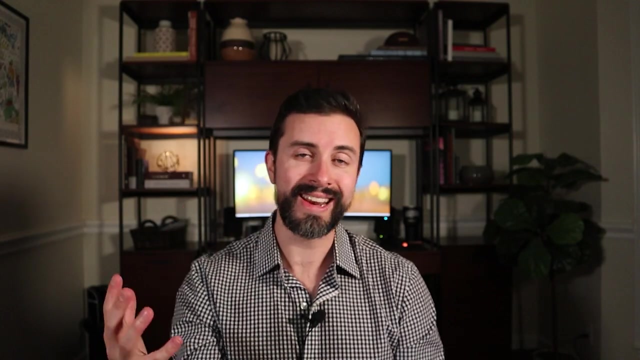 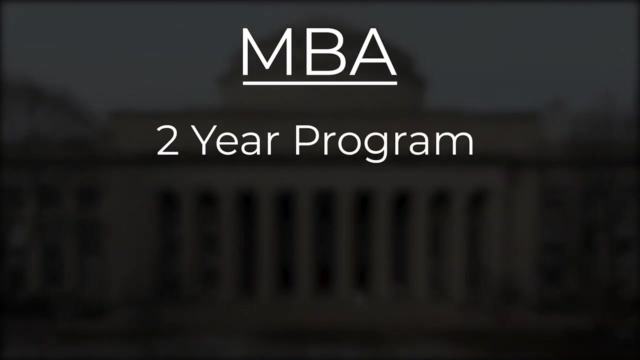 average salary expectations. we also do really need to look at cost and also time to completion. That is time to complete the degree. All of these are very necessary elements in any kind of ROI calculation. An MBA from MIT would take approximately two years to complete and tuition. 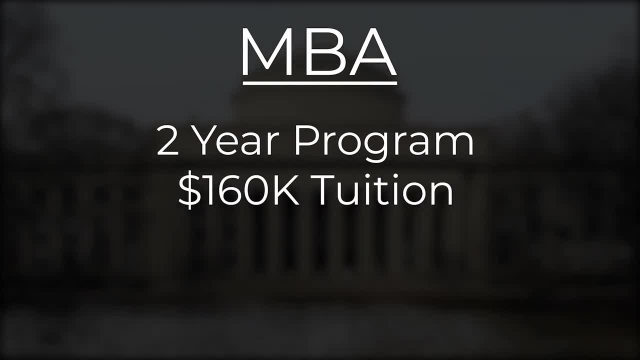 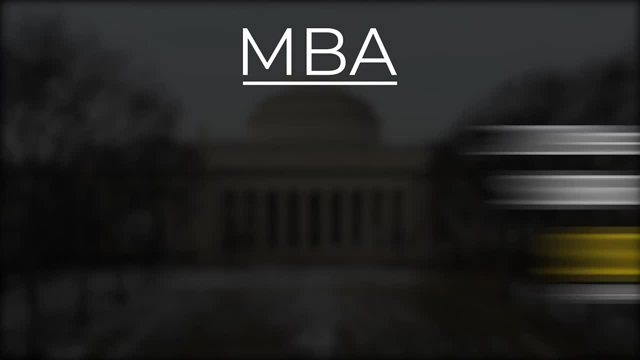 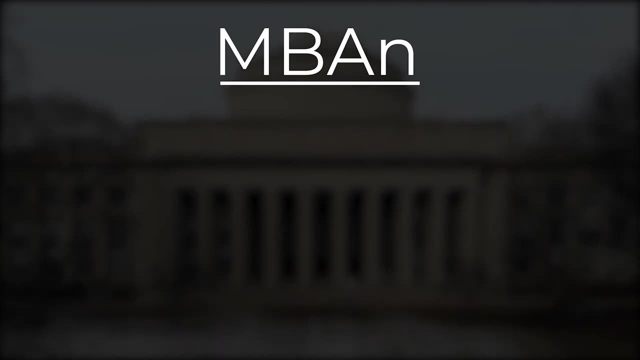 alone would be around $160,000 for the two years. Average base salary is 148,000.. A master's in business analytics- in the case of MIT it's called an MBA, lowercase n, presumably for analytics, because the acronym is could actually be the same. This would take about one year to 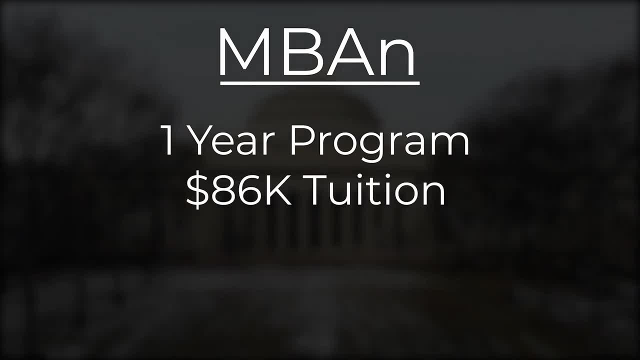 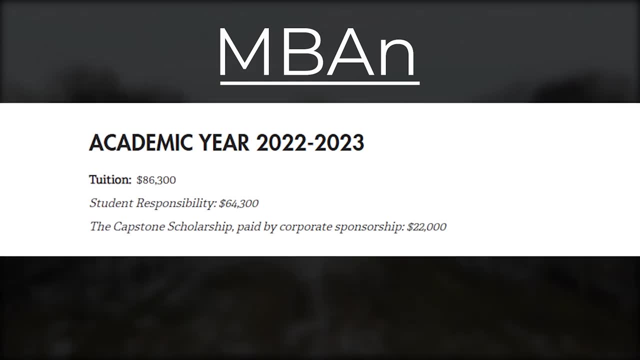 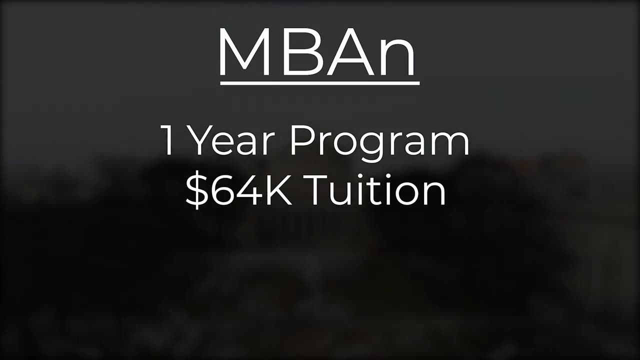 complete Tuition would be 86,000 for the program. But 22,000 of that is actually paid for by company sponsorship through a capstone project you would be doing towards the end of the program. So really your out-of-pocket tuition costs would be just $64,000.. Average base salary coming out of the 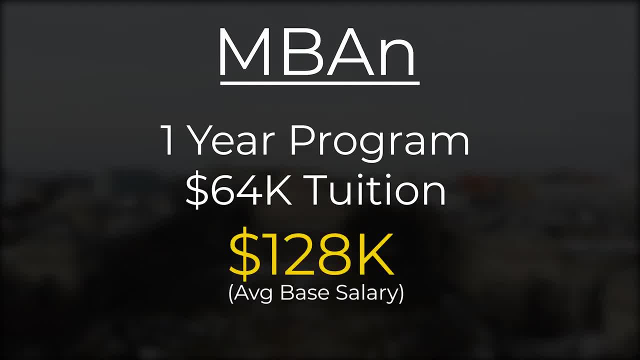 program is $128,000.. So about 20,000 less than an MBA. So, in comparing these two routes, granted, it's an MBA, it's a master's in business analytics. it's a master's in business analytics. it's a.